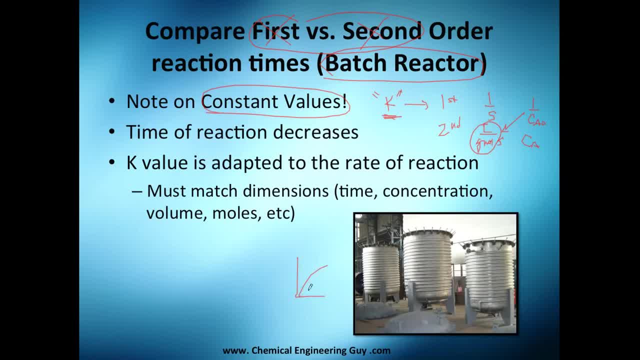 later, hopefully in next chapter. So you get that constant is essentially experimentation and when you experiment you just go like this: Whatever you get here divided by whatever you get here. Sometimes you get seconds, sometimes you get even more complex stuff like c of b concentration grammo to the third power. 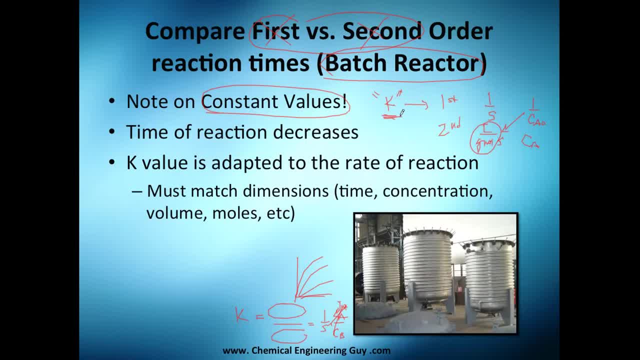 whatever. So just keep in mind: k can or may have any value here: Grammo, square grammo to the third power, liters, Even square root of liter, which doesn't make sense. but I'm telling you this comes from experimentation, So just trust in me and you will get the concept. 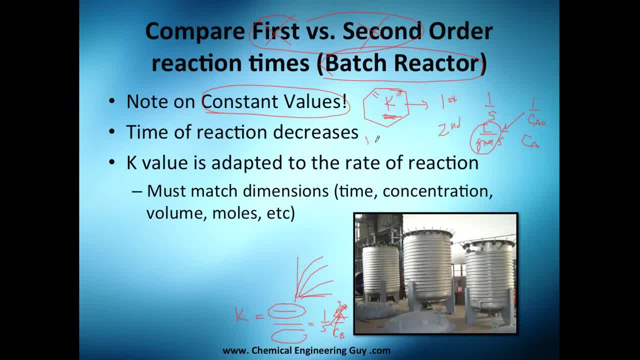 Now the time of reaction decreases in the second order. So maybe you remember was six hours for the first order and 2.5 hours in the second order. Why? Well, first, of course, it's because of the mathematical model. What we want to do is actually see that our rate of reaction depends to the second power. 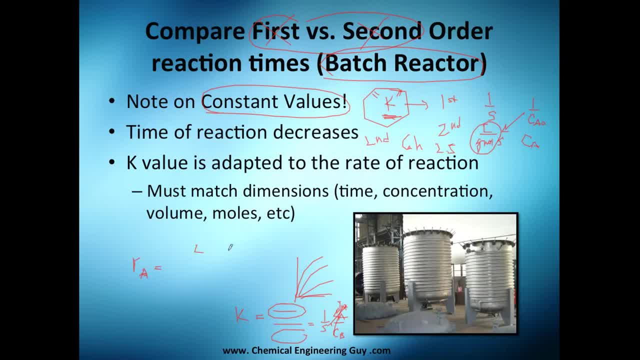 So as concentration decreases, you get lower and lower and lower rate of reactions. Lower rate of reactions means the reaction is taking actually place. Now the k value is adapt to the rate reaction. Okay, yeah, that's what we were talking about, And let me continue. 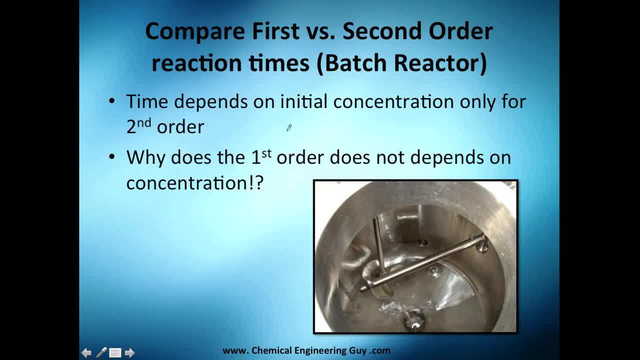 The time. dependence on the initial concentration. I love this exercise because it's Ca0, or initial concentration. Let's say it could be 10,, could be 5, could be 1 or even 0.1.. The thing here is that in the first order reaction, you will have no problem at all with this. You can. 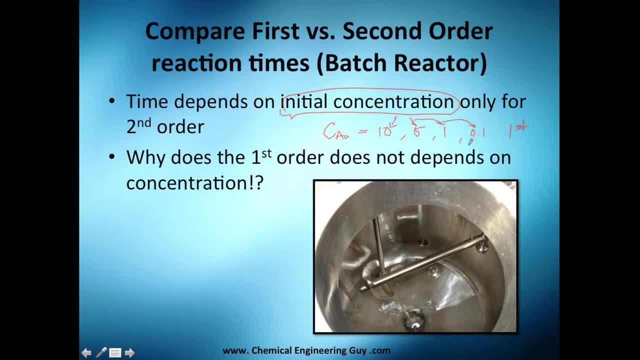 have different initial concentrations and the time dependence on the initial concentration. Let's continue The time dependence on the initial concentration. I love this exercise because it's Ca0, or initial concentration. The time required for that will be actually always different? No, always. 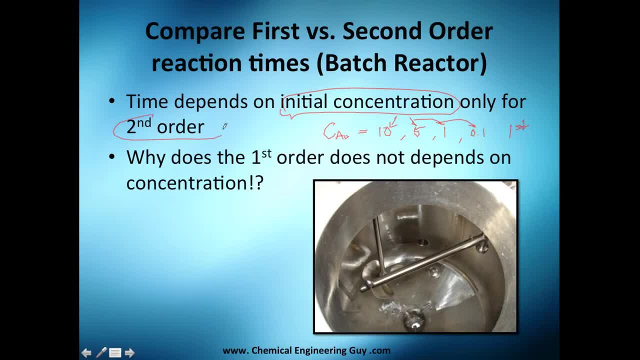 the same, But for the second order reactor. you have these concentrations and you will see that you actually have a change in Y, because you got this kt and I remember 1 minus X. I think this was our time for second order. So, as you can see, as Ca gets higher, 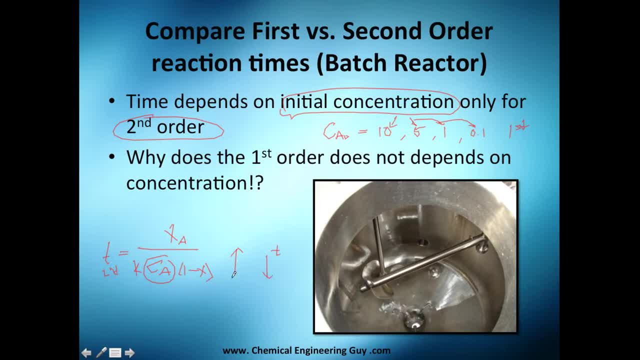 then you get lower times so you want higher concentrations at the beginning. so i remember when i asked this in my, let's say, class and my reactor engineering and i think also energy balance, and i asked my professors and they told me that they they could not explain it very well, like 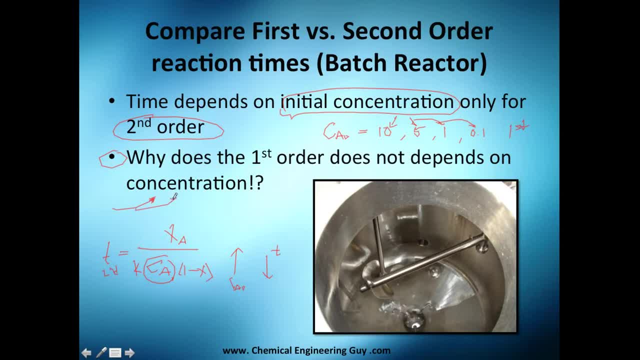 it was more about about mathematics, and i do agree that it's about more in mathematics rather than in actual physical concepts. i could not explain you guys why, physically, a first order reaction doesn't care in the initial concentration. i can tell you why mathematically, and i know. 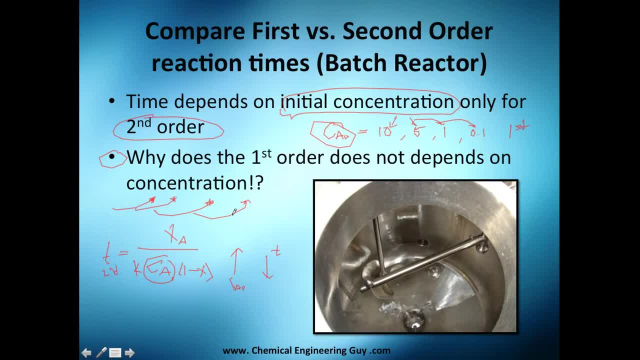 it, but i do not. i cannot explain you guys. so hopefully you get this question with your teachers and they might give you a better answer, as i did. but worst case scenario, you do know it does not depends on the initial concentration. that's very important, and i want to also tell you the procedure with it. 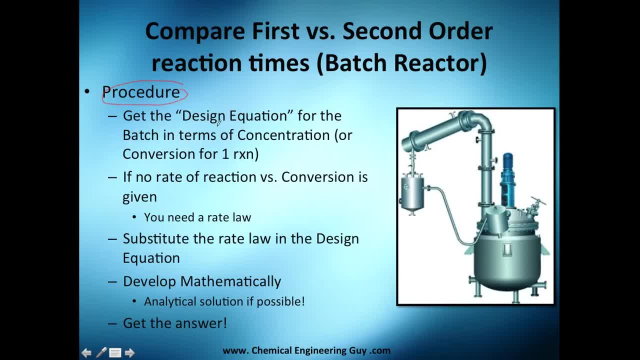 because maybe you saw the methodology and you never saw it applied, and the thing is that we actually do use that methodology. so the first thing we did was get the design equations, which is dca divided by dt equals r of a negative and negative in terms of concentration. 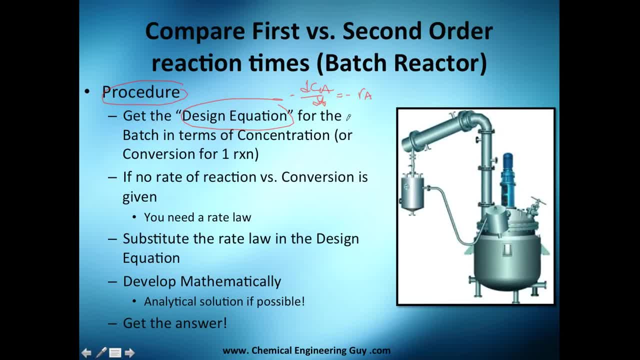 or if you're using a conversion or one reaction, you should get it in conversion, which was dx. i don't know well, actually it's before, but that's the first thing if no rate of reaction okay is given. so we weren't given the any data they just told. 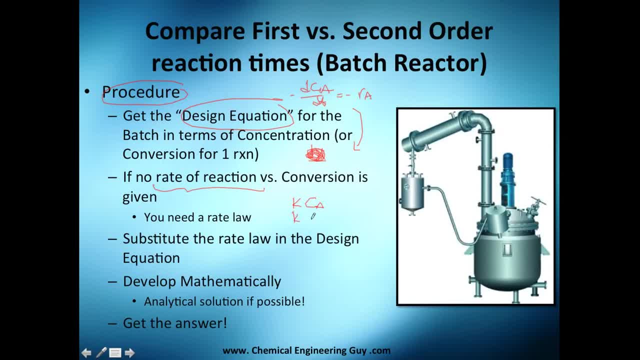 us the law, which was this for first order and this one for second order, versus conversion. yeah, we could, they told them. they never told us that at x value you got this rate and at x different value you got this different r of it. no, they didn't actually tell you, so we 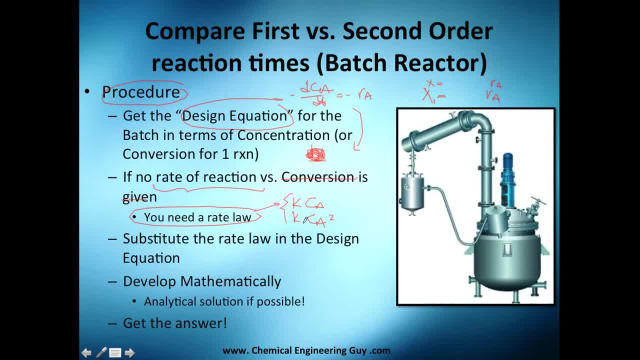 need or needed a rate law, which they gave us, so it's fine. then we just need to use the design equation found in this here and the rate law here, combining mathematically, and then we can start developing these equations by math. you will get the analytical solution if possible, because sometimes you get. 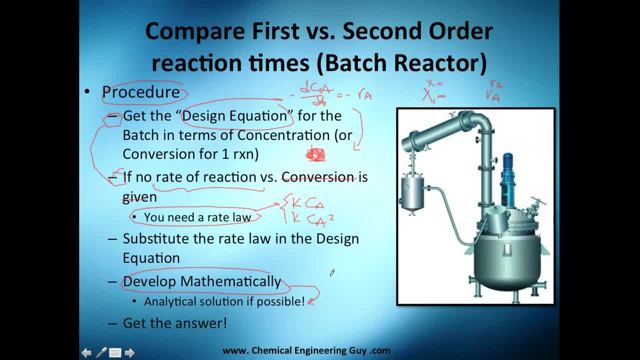 like crazy stuff with differentials, and you will need to know how to solve them, or at least how to use a software that solves it. and well, eventually you will get the answer, if you did it analytically, or if you did it by numerical methods, or 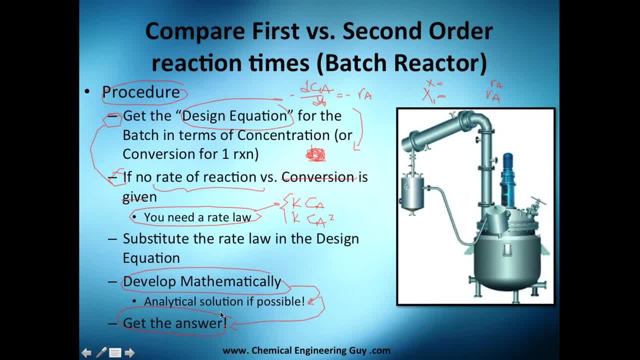 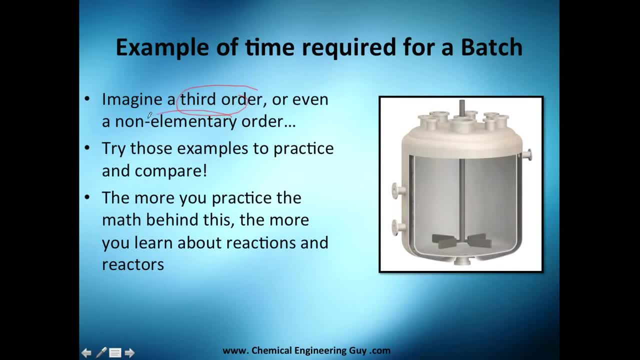 with a computer. the important thing, of course, is to get the answer, and this is for you guys. imagine a third order, or even a non-elementary order, which is very common cea. imagine this rate of reaction. if i tell you this rate of reaction, how would you solve it? 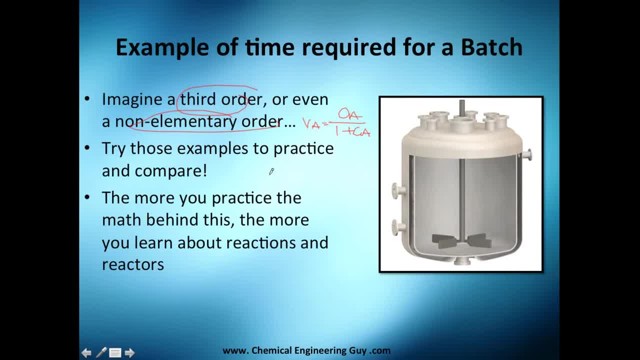 uh, just think, try it at home, homework and compare them. of course, comparing is the best thing that can happen to you, because you can get to see different cases, and when do you get more problems or troubles, or you? and yeah, essentially it's always good to compare the more you practice the math behind this, because 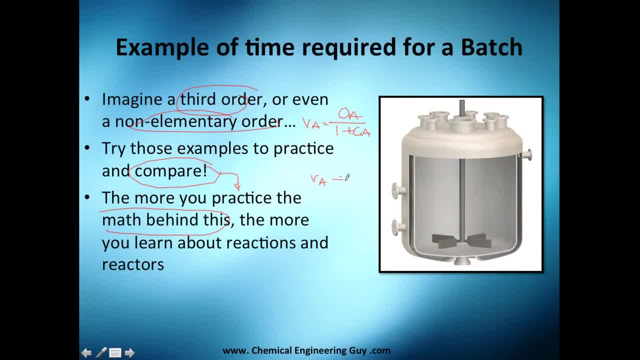 i know the theory is the same. you just put the rate of reaction in the equation. but what happens when the rate of reaction is like this? or what happens when you have only k and has no dependency on ca? or what happens when you have c, b? all those kinds of problems you will need to know. 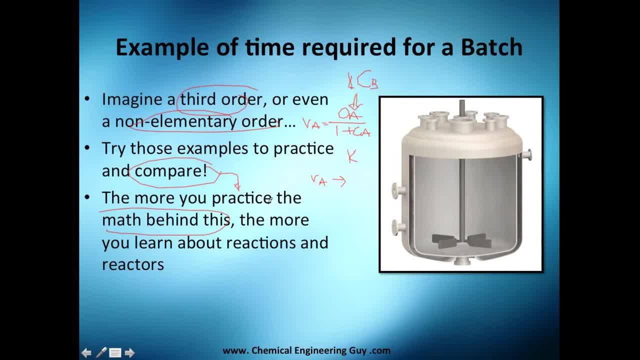 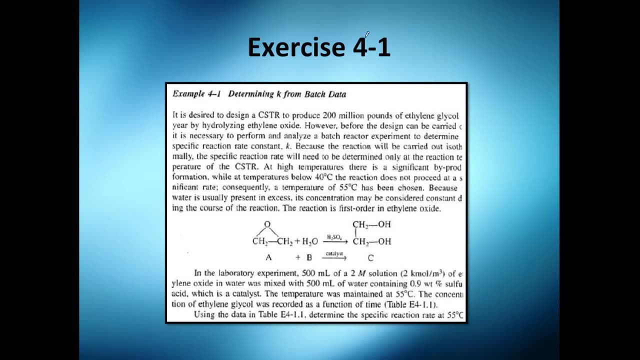 and are not shown here, and also in the books, are not shown that much. it's not. you need to practice and question yourself. so this is better, because the more you learn, you will learn reactions and reactions. so it's time to do exercises. actually, this one is from the book. uh, you want i'm going. 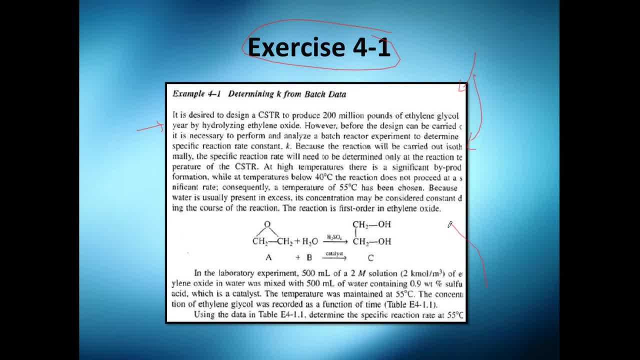 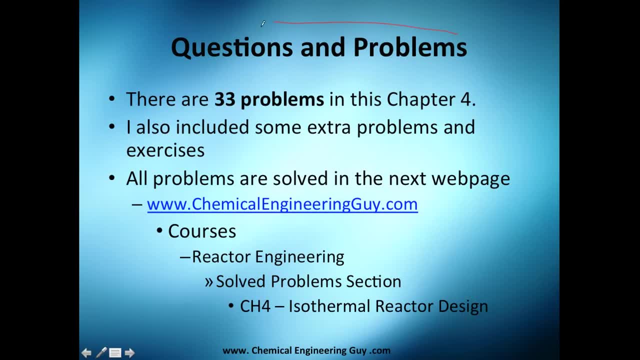 to solve it and upload it into the course. so if you want to check it out, just go to my web page. actually, yeah, i have this link in the description. i always put this slide because i have individual videos, so you have got more extra questions and problems. you can go there. if you check your book, in chapter four you have three true problems in 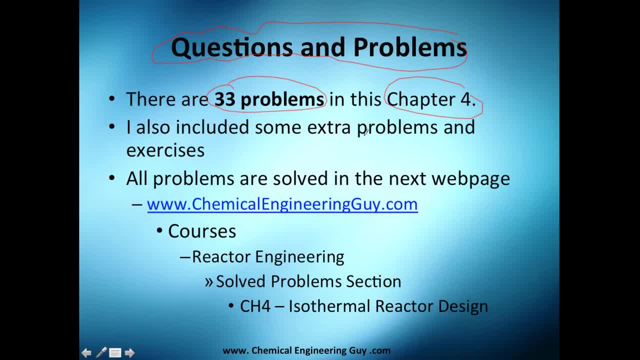 the back side i also included some extra material problems, pdf word materials, recommended articles, many stuff that will help you. and if you are interested, you can go and check out this web page, go to the courses area react engineering and then click in the solve problems section. then you will probably check or see that. 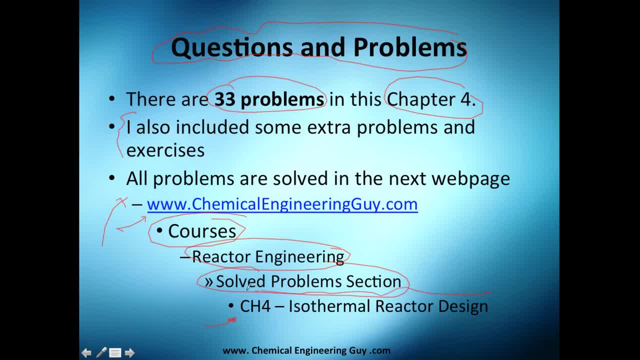 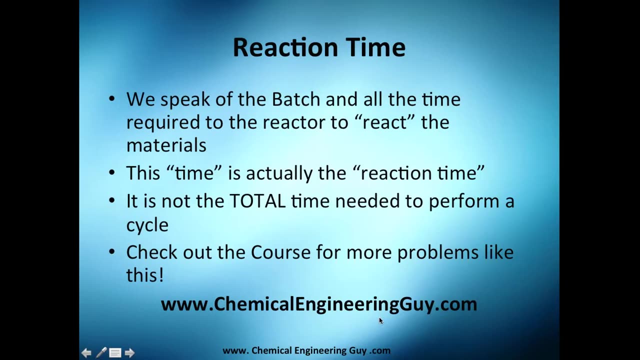 you have some chapters. go to the chapter we are right now, which is chapter four, is a terminal reactor design and i will be popping or uploading the the videos here. so the next topic will be reaction time and i think i'm going to break the video. see you in the next one. 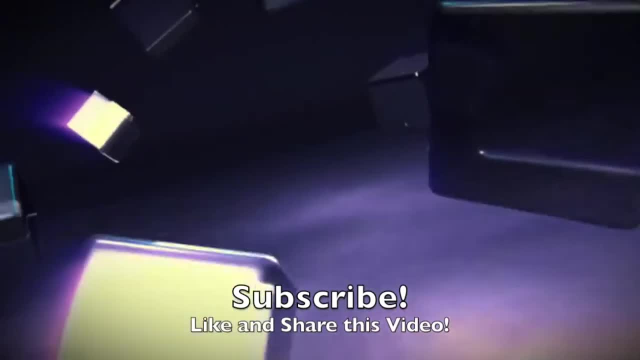 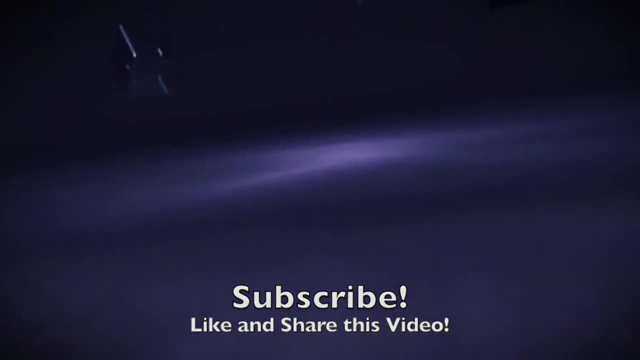 what's up guys? it's me chemical engineering guy. so if you like the video, why not push the like button? it really helps me to know if you're liking the videos or if i should be changing something or i should be adding something. taking out content, whatever. also, sharing is caring, so if you got any, 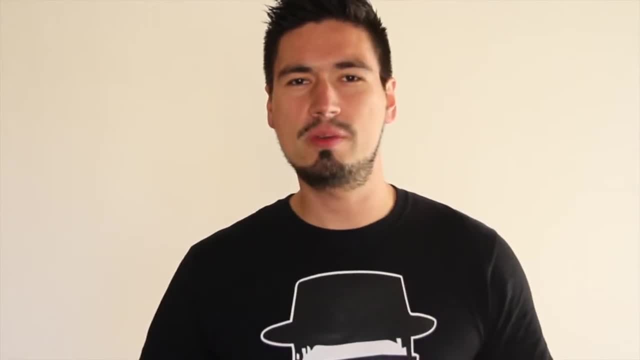 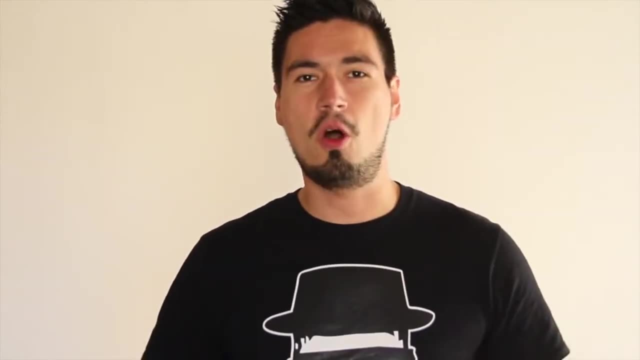 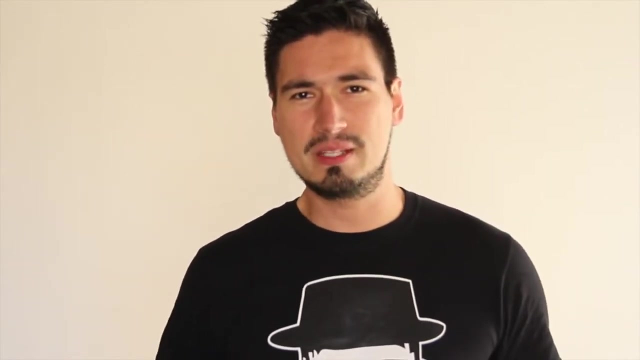 kind of friends, teachers, colleagues, friends or whatever you want to share with me. i will be happy to share it with you and i will see you in the next one. bye, bye, or whatever kind of person that might be interested in this type of content. why not share it? sharing helps our community to grow faster- in members and in content. 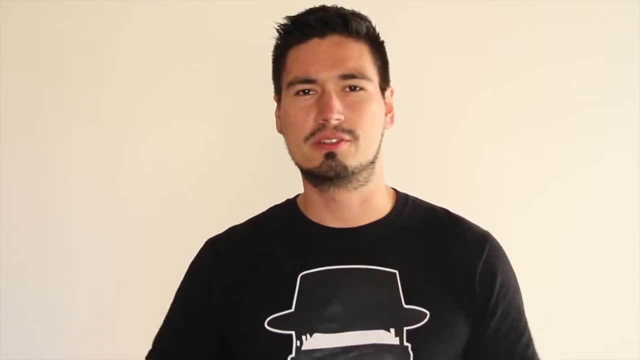 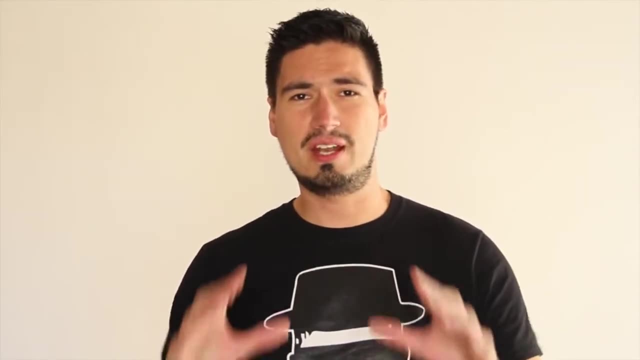 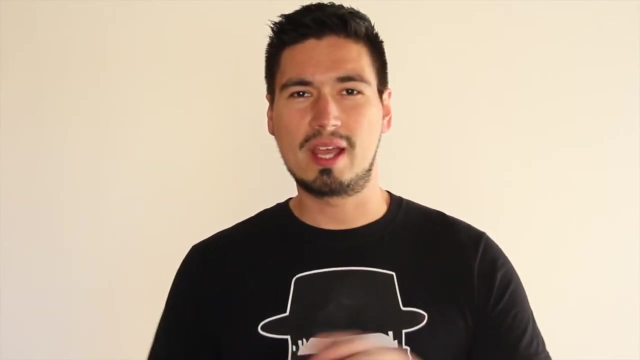 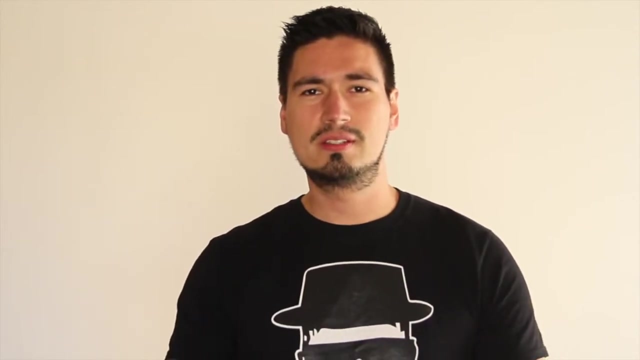 if you want to keep track of my activity- videos uploads, experiments, plays, whatever content i'm getting youtube- be sure to click the subscribe button. subscribing to the channel is totally free, guys, my dream is to create an online academy of chemical engineering where everyone can access it in the world. imagine a place in which the student, the teacher and the engineer get. 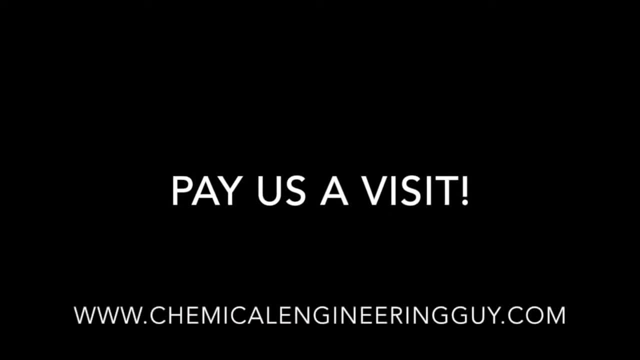 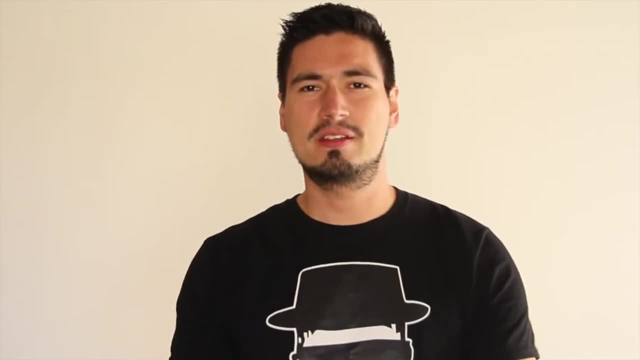 the best of each other. so thank you, thank you, thank you, guys, for the support and the love.